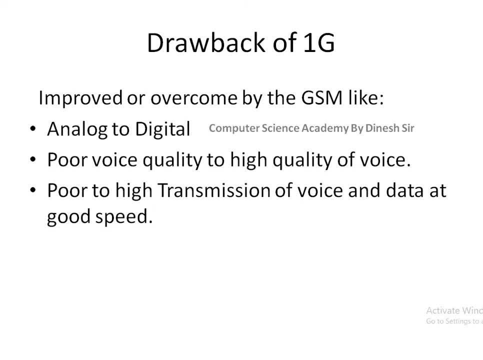 First one, in the zero generation and first generation analog communication was utilized, due to which the voice quality was not good. it was pure voice quality and it was overcome by the concept of GSM. And, yes, the data transmission speed was also very low. there was no internet. the internet was also launched by GSM when that concept was launched. 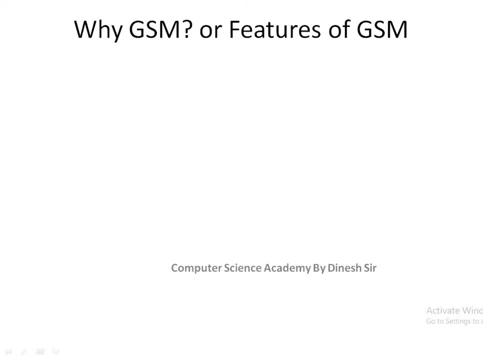 So, first one, what is GSM and its features? So first of all, we see what is GSM. GSM is one of the key features of the GSM. It provides the high quality voice and data services and daily communication. Why did it do all this? 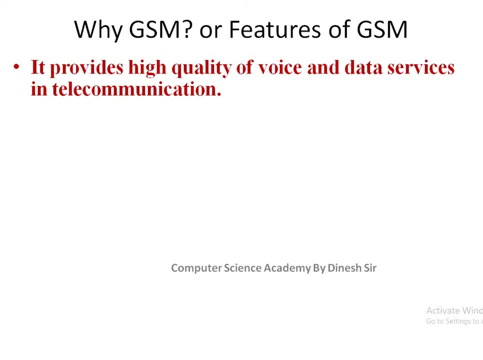 Because the first generation mobile phone used to work on analog signal. but when the zero generation technology came, GSM technology came. so what did they do? They replaced the technology of analog signal with digital signal technology. So due to the digital signal technology concept, the voice quality improved, data services were provided to customers at a high speed and even roaming conditions were also done. 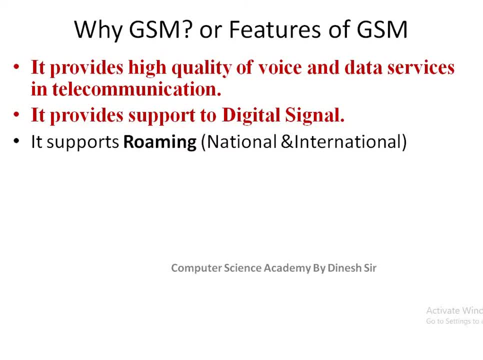 Means a person can move anywhere without changing the mobile number, So this concept also supported it. A feature was included in mobile phone communications that it also launched the roaming concept. It provides high quality speed voice. The data speed is also very good And its base station means the tower was of high energy consumption. 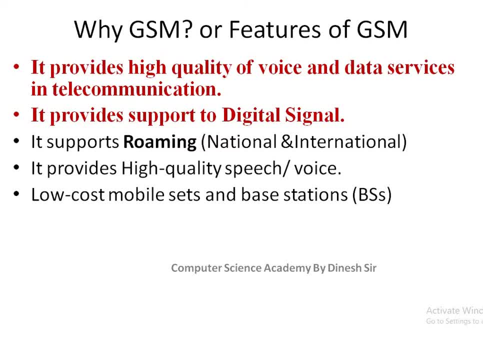 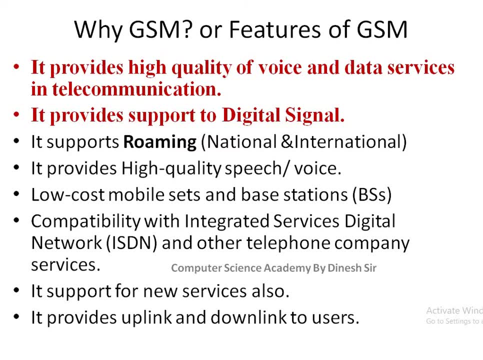 Now low power consumption antennas have been mounted in it. Now integration is also compatible with any network at any time If the user is switching from one place to another. if the user is in a roaming condition from one place to another, then it is not necessary that he should have a similar configuration everywhere. 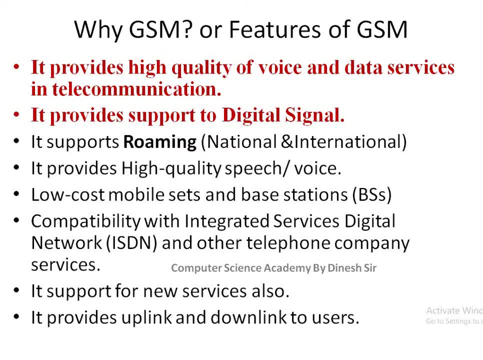 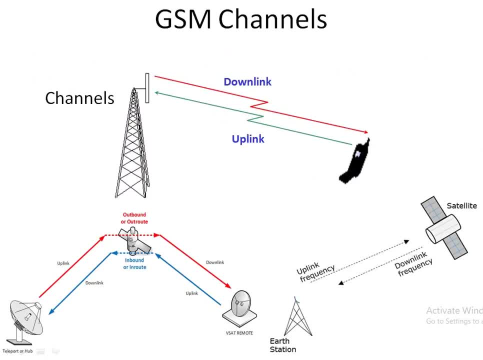 If he gets a network of similar configuration everywhere, then it means GSM does compatibility and integrity with each network. Now that is the diagram of downlink and uplink. Downlink means downloading and uplink means uploading Means when the transmitter transmits signal to us. that is known as the downlink. 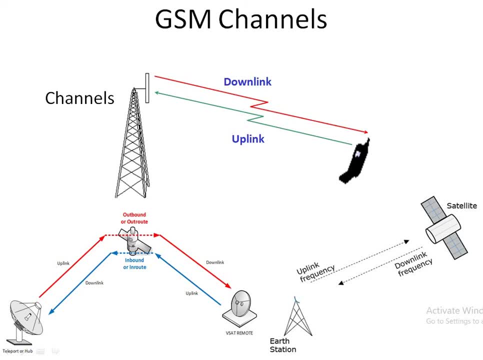 And when a mobile phone catches a particular antenna, sends something, sends voice, sends data, then it is known as the downlink. That is the uplink means uploading. Next example: the signals that we get through the satellite, the disks of the D2H receive. that is a downlink. 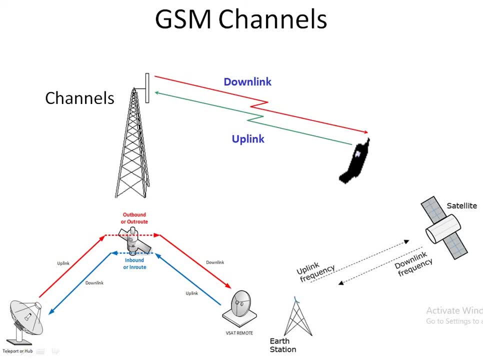 And when it is a kind of BSAT, which is in every organization, it is used to transmit the signal. So when the signal has to be transmitted, that is the downlink, And when it has to be received, it is the downlink. 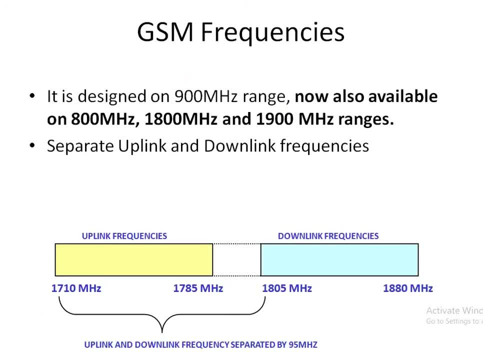 And when it has to be sent, it is the uplink. Now, at what frequency does it work? It works on the 800 MHz, 80 MHz, 90 MHz, different frequencies as per the requirement. So what is the requirement of the network of every place? 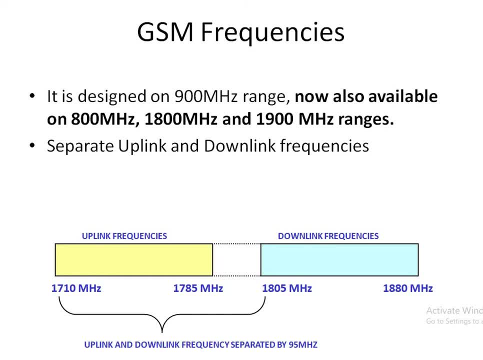 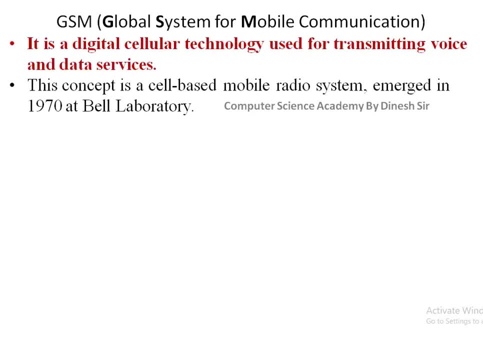 For what type of design is it done? It depends. If we talk about it commonly and generally, then it supports on three frequencies. GSM is the Global System for Mobile Communications. that is the Digital Cellular Concept, Means in the 0th and 1st generation there was analog technology. 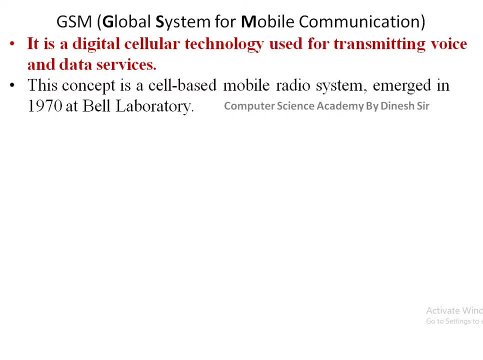 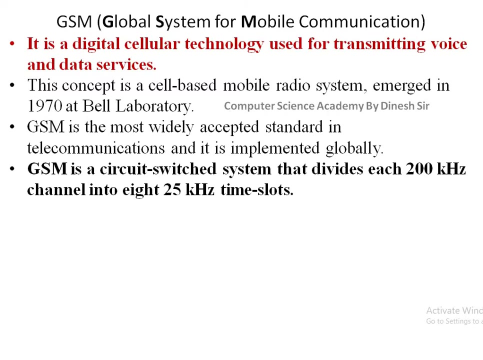 The second generation onwards. the digital cellular technology concept of GSM was launched and developed by the 1970s at Bell Laboratory. GSM is the most valid and accepted standard And GSM is a circuit switch system. What does circuit switching mean? It means that there is a telephone in our house that is the landline phone. 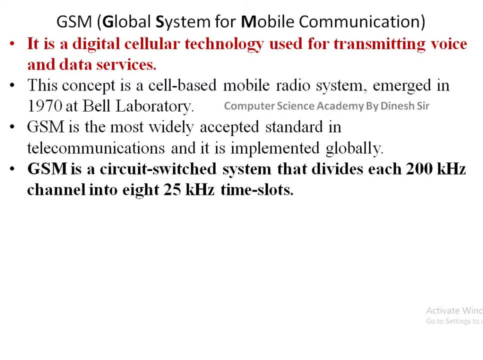 So when we connect our mobile to a physical wire that is the landline phone, So when we connect to a physical wire that is the landline phone, Our mobile phone is connected to that physical wire. that is the Digital system and circuit switch system. 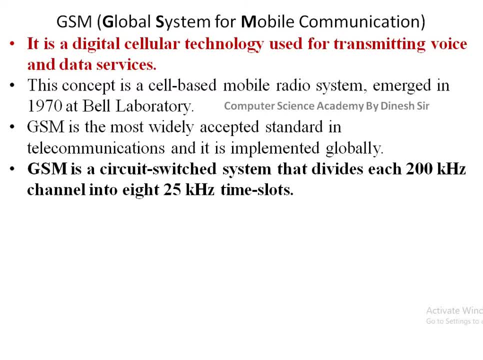 By which we are just transferring the voice from that phone to another phone. GSM makes use of time division- multiple access. Multiple access is the kind of medium by which all the signals are transferred from the user mobile phone to the tower and mobile switching centre. 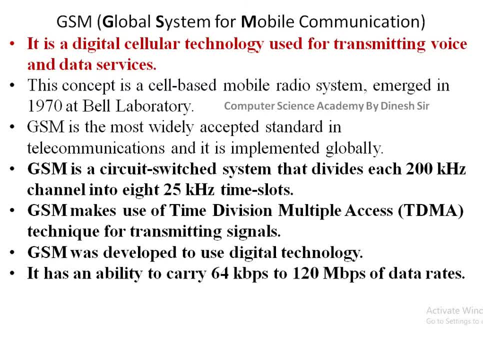 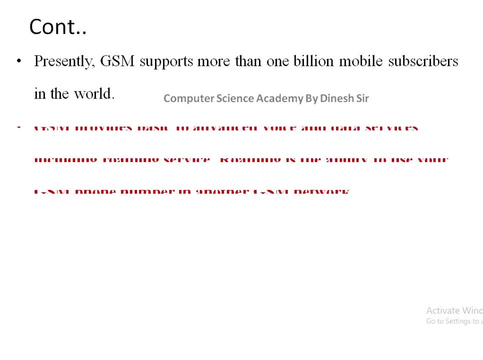 GSM is the most valid and accepted standard GSM developed to use digital technology and it provides a good high-speed- me see a 64 kbps to 120 mbps data support. it's called support cut. that means a high speed data transfer connectly support cut. that next one is the GSM provide, the 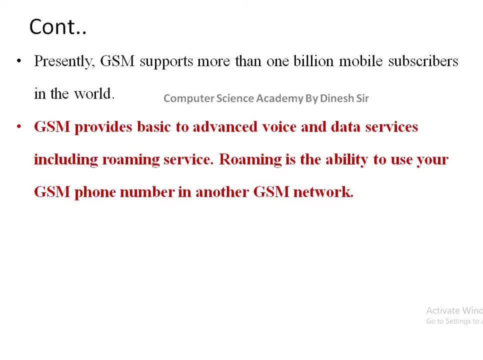 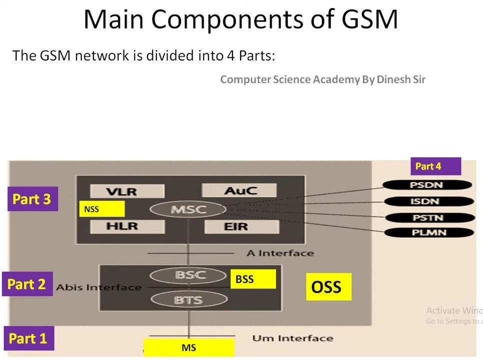 advanced voice means. advance means means voice quality is more too much, good, too good. GSM operation, the different, different frequency, as we have already described. that is the diagram of the GSM. GSM diagram, each divided into the four power. first, one part is the MS. second one is the part 2, that is the BSS. third, 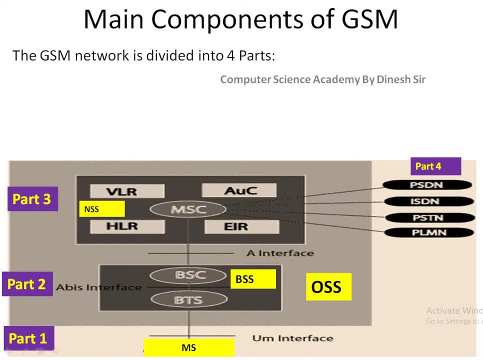 part is the MSS and fourth part is the OSS. so these are the four component of the GSM. so what is the 4 gm? mobile station? mobile station, all of us, i am all love mobile phone phone. leke chaltein, carry karke chaltein to mobile phone. hi koi, mobile communication terminology. 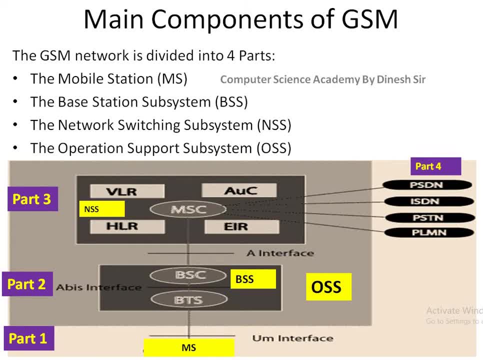 mein mobile station boltein hai mobile users. base station subsystem: kya hota? base station subsystem is the combination of the two things. first one is the bts. bts, kya hai? tower hai, antenna hai. aur bsc, kya hota bts ke sath, jo ek operate karta hai antenna aur tower ki? 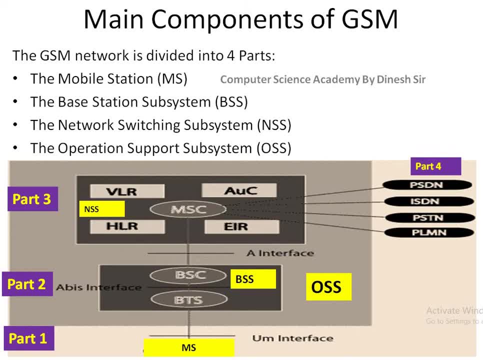 functionality ko smoothly functioning karta hai, governed karta hai. that is a kind of centers to base station controller. ek kind of controller hai tha, jo ek particular tower ke liye, ek smoothly functioning karne ke liye proper kaam kar raha hai ya nahi kar raha hai. 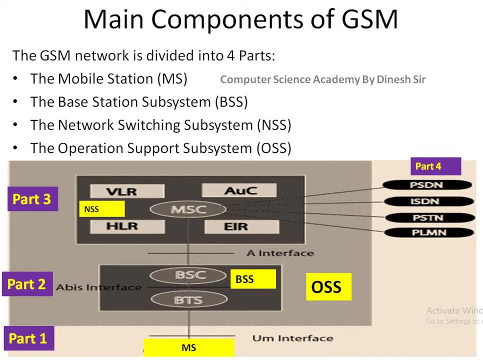 so that is known as the bsc. bsc is connected with the msc. msc is the third part and whole sole responsible for all the communication. that is, the part 3 to msc jo part hai iske, and the msc is the mobile switching center or mobile station controller, ab iske paath. 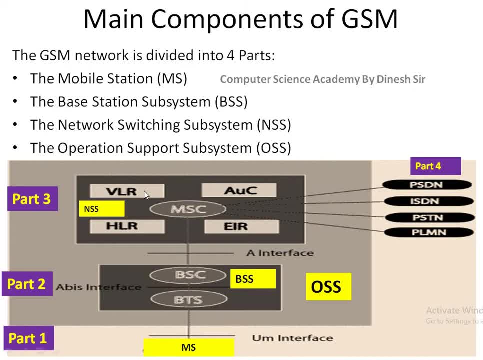 bohut saare iske sath add on features rehte hai hai. so in this case, what is ok? so municipalities ko understand saari bete hai. yea, yeah or whatever. theseön je as a user belong karta, subscriber, belong karta blr coming in with a suppose. 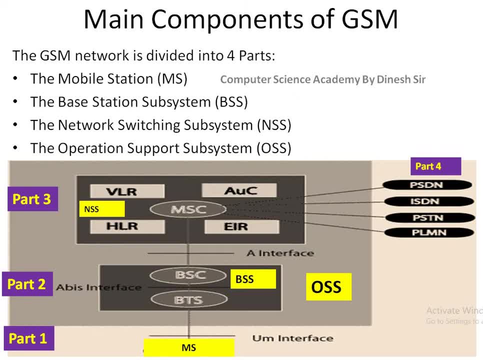 medalli second year to see the move car route to marry your location. switch we to location case a Pata chalegi will be a lark, a throw. Pata party blr is the kind of register that provide the information about the particular user, whether he is moving or where they are moving or not, the just particular nice. 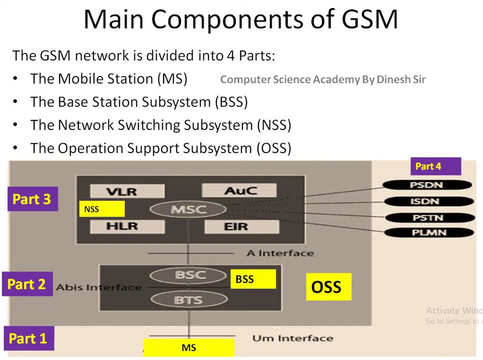 a gap, a giant- it was capacity or a user can mobile phone may either welcome to Karnataka State, welcome to Maharashtra State. page or nice statement will change. move Cara to Jesse Oski. location change with a welcome, a message at a authentication center. chaotic authentication provide karta. a kharik device could check karta. a couple mobile network may have valid. 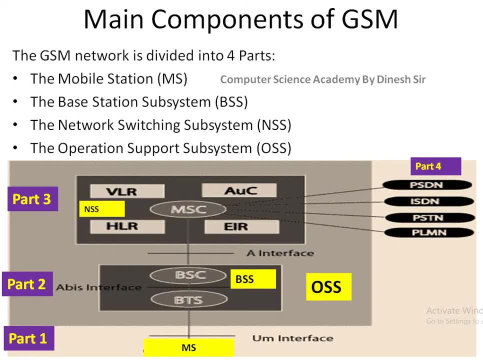 hair or not valid are getting a little person. I'm, but I'm a bell. it means a parquet or equipment. identity register means kota. mobile phone can break. I am me. I number of the disc atro a. that is a kind of physical address of a mobile. 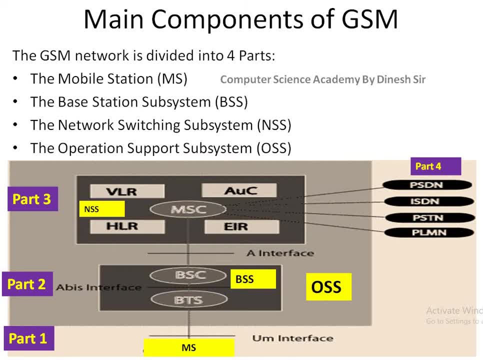 device. so that is the equipment identity register then, by which we have to trace out the particular user. this, in mobile phone, could easily track carcass. a pair of fourth part is the PSD and PSD and PSTN or PSD, and kya hota a, that is the external network. kota, just get through amara, a network come karta. 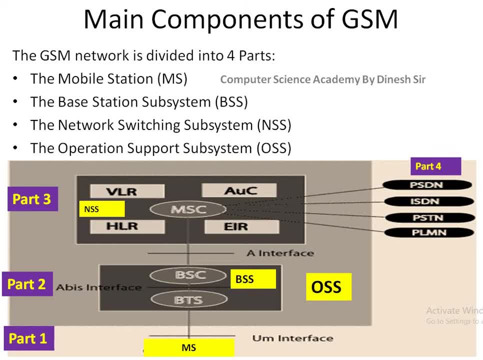 govern karta suppose a be of daily matter. daily k pura a tino part daily me, hey, or a kiss, a connected raga, three uske telephone exchange, a connected raga or a job. amari ko be called in morrow, let will say cado. 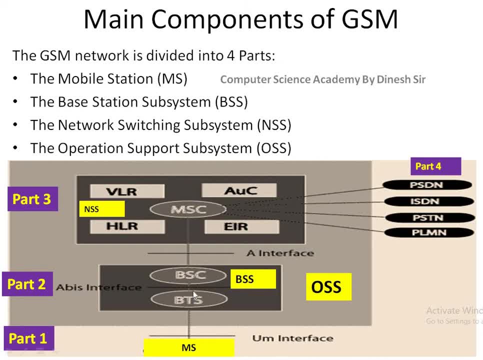 karta cvr havada for me, and then I need your buzzer. okay, Dave, happy htm Kebar Rubber, or go out here for part cao kar pass with a risk andORY charitos are common if or parts of kura h Xuara diagram divided. 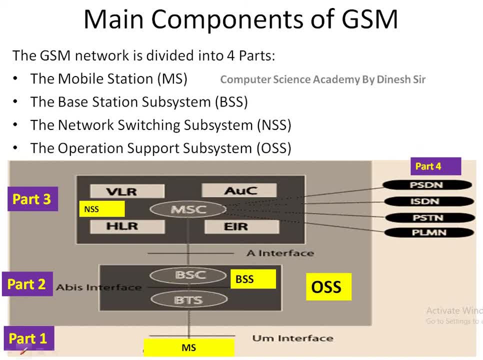 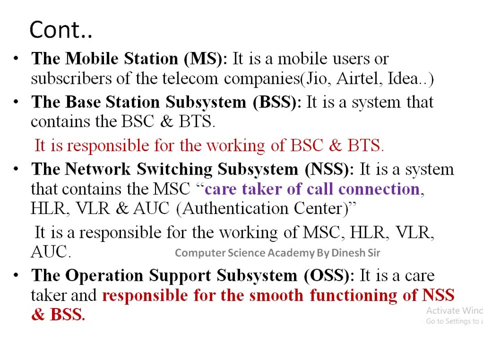 mobile communication. four parts were divided at. the first one is the MS, second one is the BSS, third one is the NSS and fourth one is the OSS. OSS means means the combination of BSS plus NSS, now the BS. what is the mobile user? BSS is the combination of this. 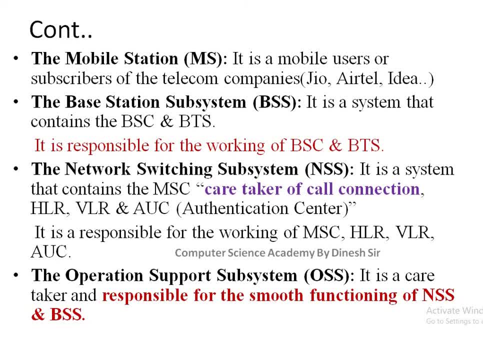 BSS is the responsible of the tower, particularly smoothly functioning of the tower. NSS is the caretaker of the call connection and authentication. and OSS is the operator support system- operation support system. it is the responsible for the smoothly functioning of the BSS and NSS, now the additional component in the 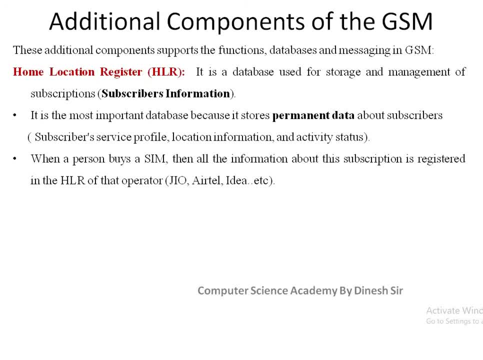 GSM. first one is the HLR home location register that provide the user information, that is the kind of permanent information. okay, which particular telecom company, which subscriber you have taken, which SIM. that is the meaning of the HLR that you are a subscriber of Jio SIM or 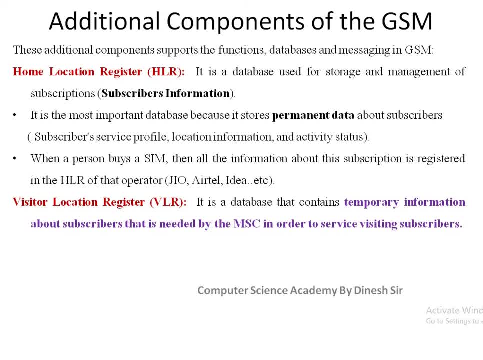 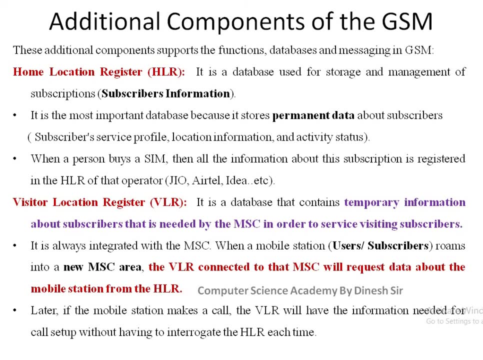 subscriber of Airtel or subscriber of Idea. what is BLR? what is the digital location register? whenever you switch your location, move from one state to another state, so that is that is stored: the temporary information that the visitor has come to particular states for some time, so its location has changed for some time. 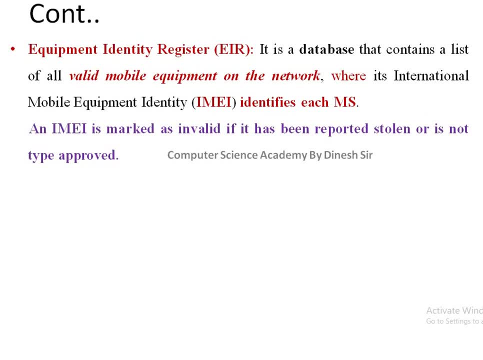 equipment identification, security, authentication and an example instantly and the phone is quickly going to be connected to anarnos. okay, so basically this fellows mobile phone taken only when they are able to reach the mobile medical facility, and usually over that number is unique because no one is able to touch it. and then it is found that such a mobile phone or phone in the digital system is obstructed from reaching the access point to the device stuff. then it gets lost easily. When a person who steals the phone would do that, and when he puts a new SIM into that with specifying him, and then what happens? that what happened will enable it and it is easily taken over and easilyライzed from there. and whenever other people will put a new sim into it, the sim pin hole in it, the guy will be put on a Sievert.